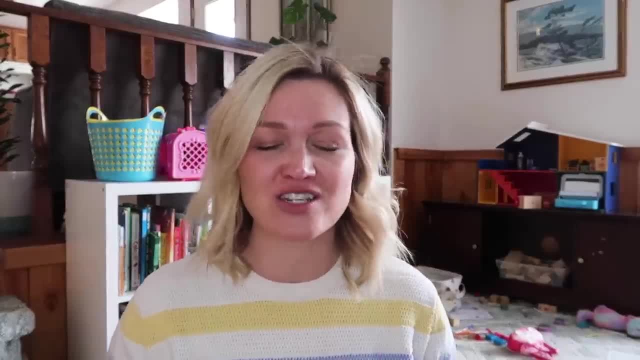 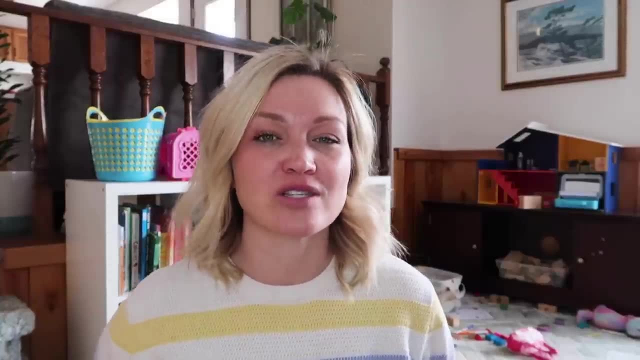 I might box up some stuff and put it downstairs to bring into our toy rotation- Sometimes stuff comes up and stays up- and then also getting rid of some baby stuff that my kids are not playing with. My son has definitely outgrown and he won't notice, So in terms of decluttering your kids stuff, 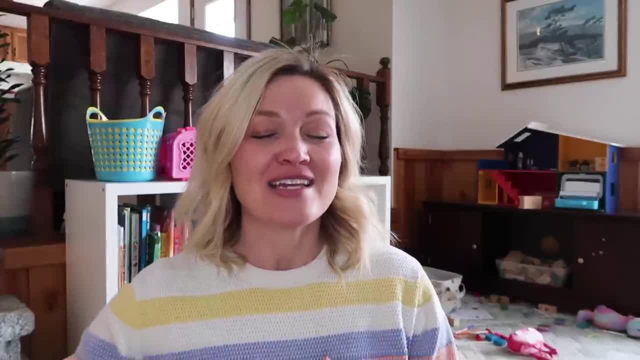 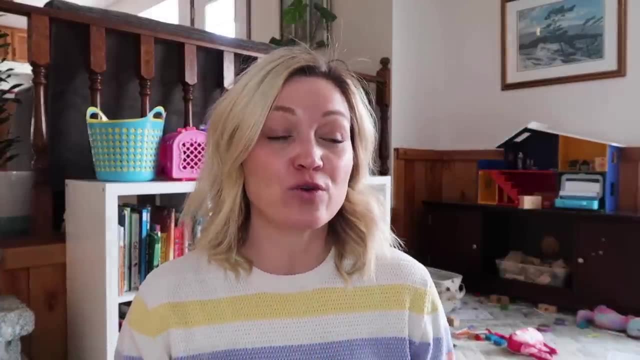 without them. I think this is very personal. There's a very fine line of when your kids are young enough that you can just throw their stuff away and it's fine. and they get old and they start getting attached to things. So if you think you're on that border, just really please be considerate. 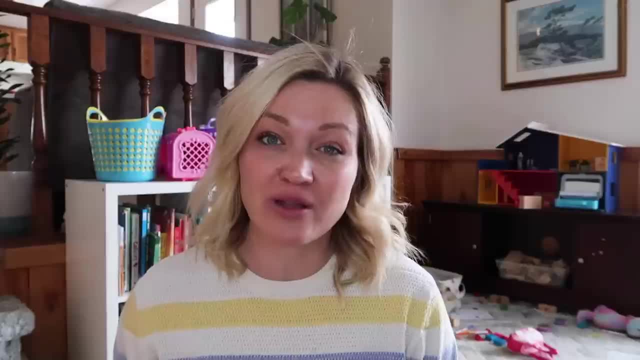 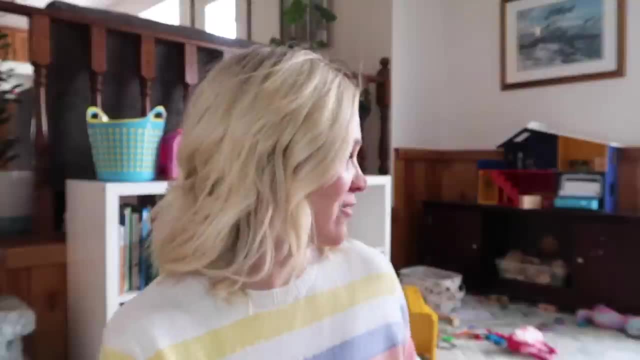 of them and their things and and maybe just ask them: hey, are you still playing with this or do you care about this? or they might be easier to get involved than you think. My daughter has helped me stuff before and she's awesome. She loves it. Sometimes she even tries to throw away things. 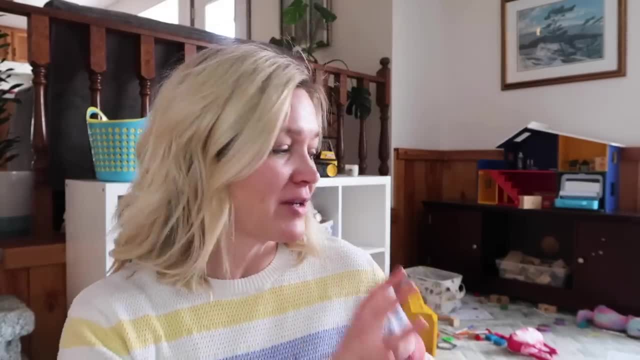 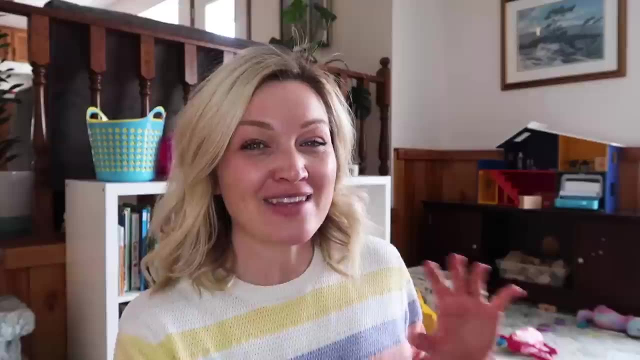 I'm like, no, don't throw that away. Anyways, I've gotten on a tangent, So I'm going to mostly just clean this up, pull some stuff into storage, get rid of broken stuff, stuff they don't like, stuff they don't need, and then baby stuff, And then hopefully just have a space here that we can work. 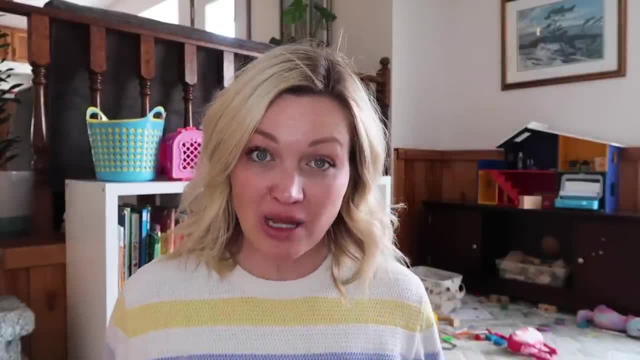 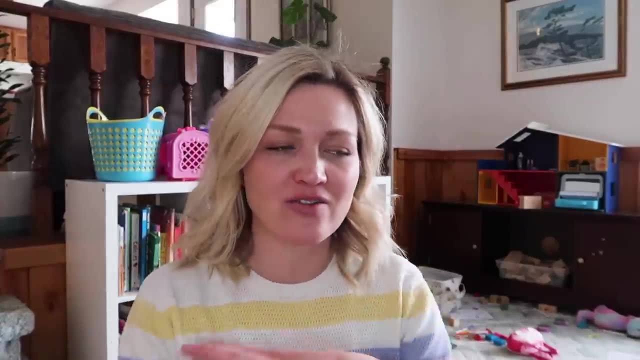 with a little easier. The other big toy in our house is art supplies and again I'm just going to go through their art supplies, get it all organized. I have to do this at least once a month because the markers and the crayons and everything gets mixed up and it's just hard to 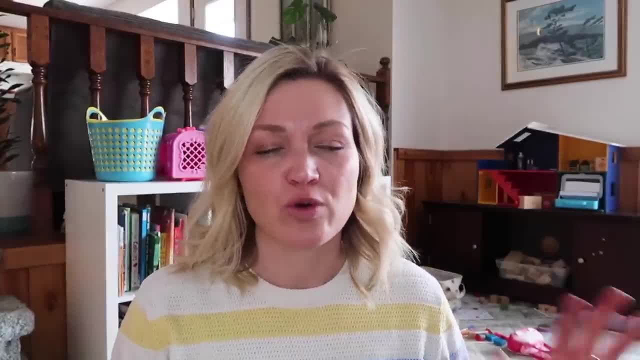 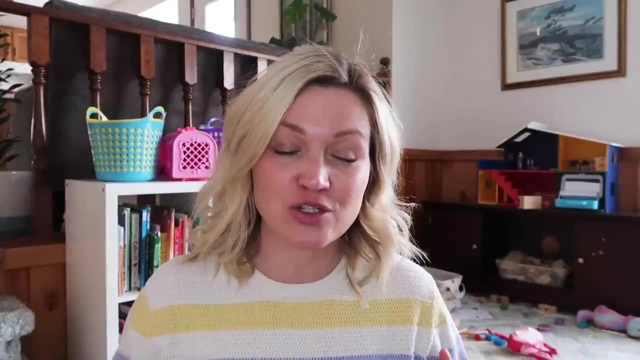 use and hard to organize. So I'm going to go through all of them and I'm going to go through and I get rid of all the stuff that's old and broken and dried up and that's kind of how we keep it organized. My kids could probably get a little more involved than they do, but we're working on. 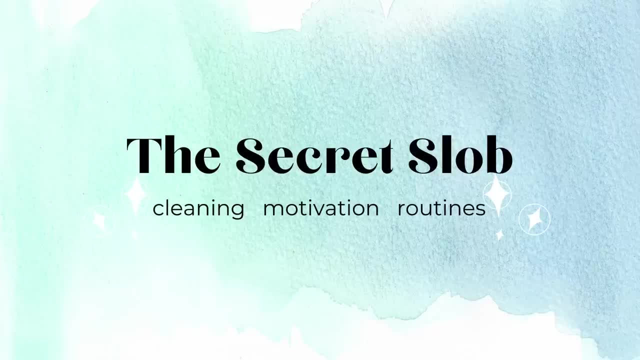 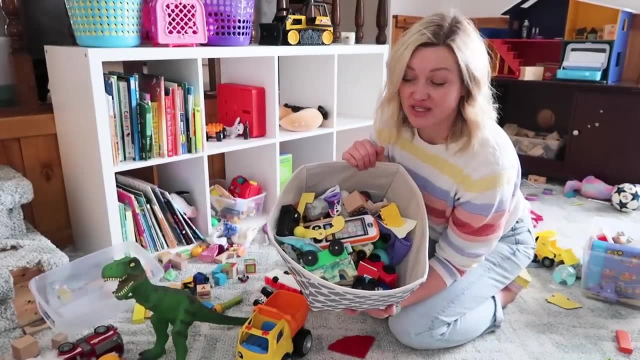 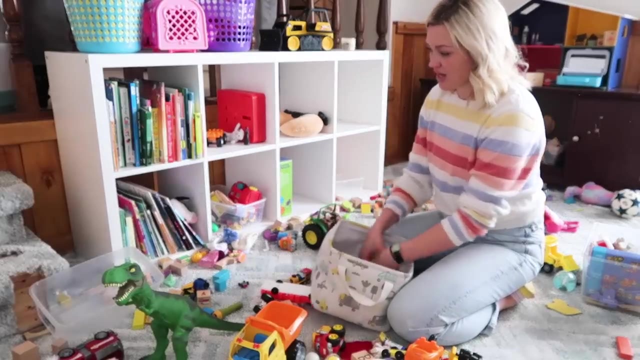 it. They're not here today, so it's a perfect day to get this stuff cleaned up. So this is our toy space Right now. it's just random boxes, So how are they supposed to play with this when nothing is even what's in here? I don't know. So the blocks are a perfect example of something that I 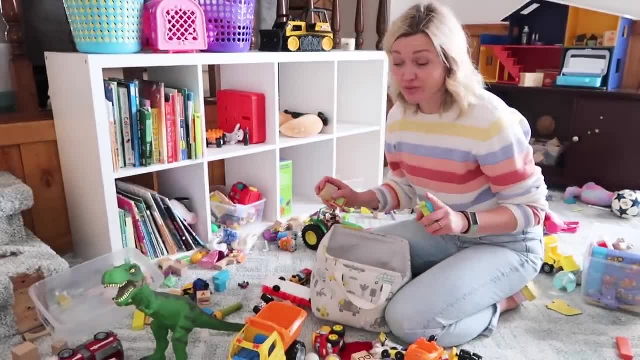 honestly want to play with. I want to play with this, I want to play with this, I want to play with this. I want to get rid of it. My kids barely play with them. They only play with them when I ask them to play with me, with them, and I'm like not a huge fan of playing with blocks, But what? 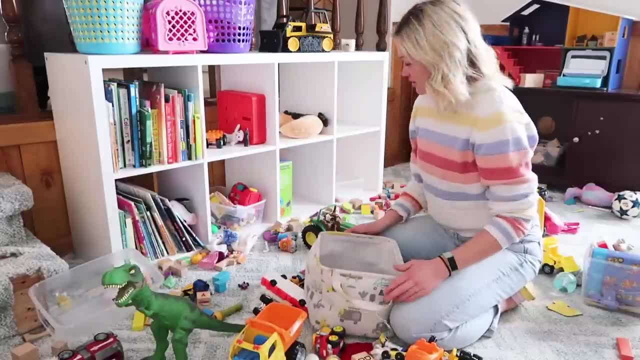 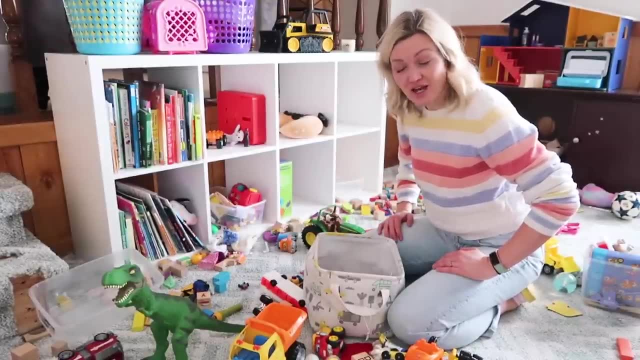 they mostly do is just take this bin and box and dump it out. So there's a really big part of me that wants to throw these away. I know it's like really good cognitively for them to play with blocks, but cognitively I feel like they're just throwing them on the floor. Maybe we'll put them. 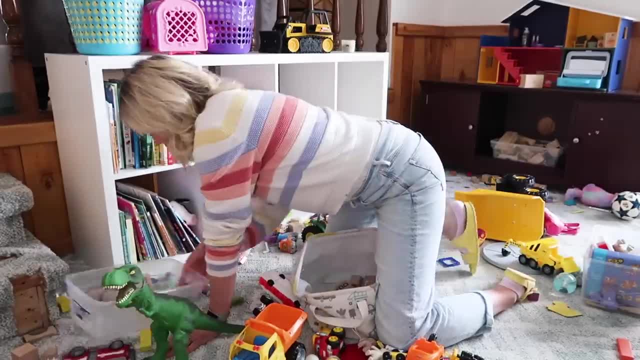 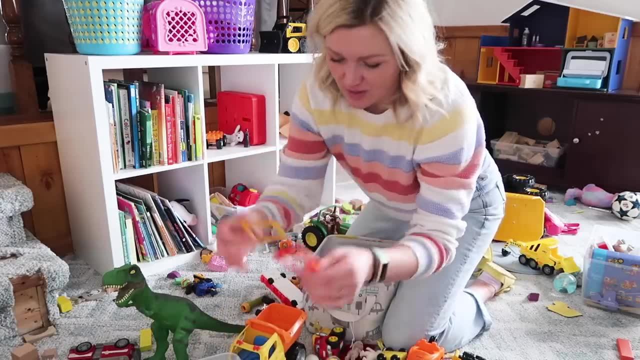 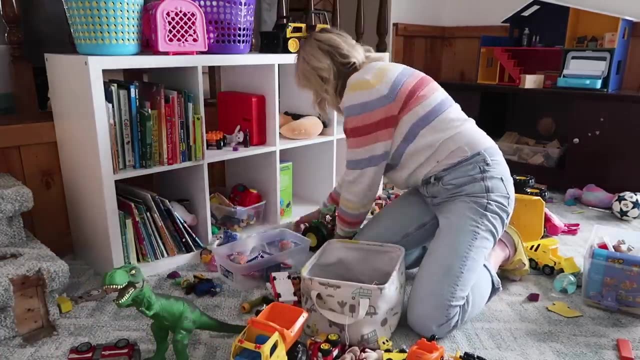 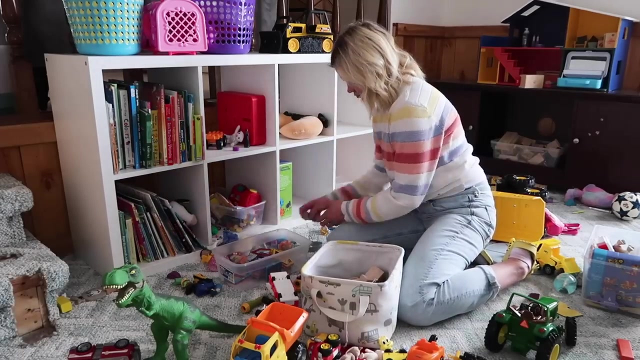 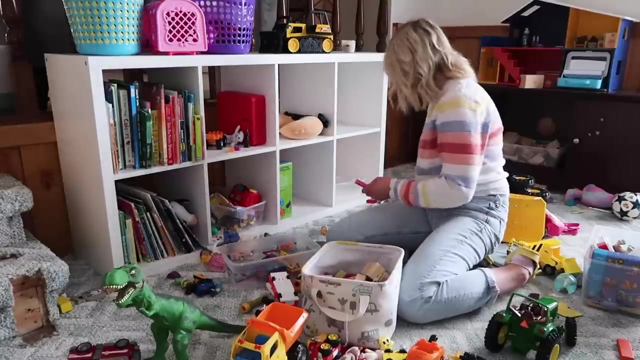 in the rotation, Bring them out later. They do like these, though, and they play with them a lot. These are these like magnet squares. We'll keep them. So blocks are contained, The magnet tiles are contained, And now it's just a lot. 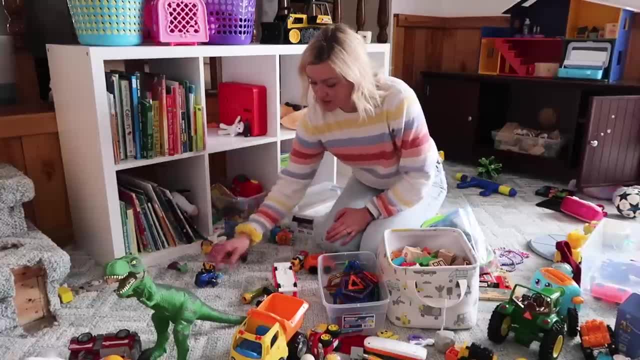 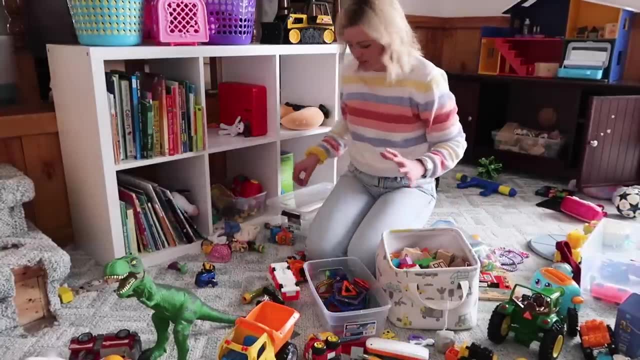 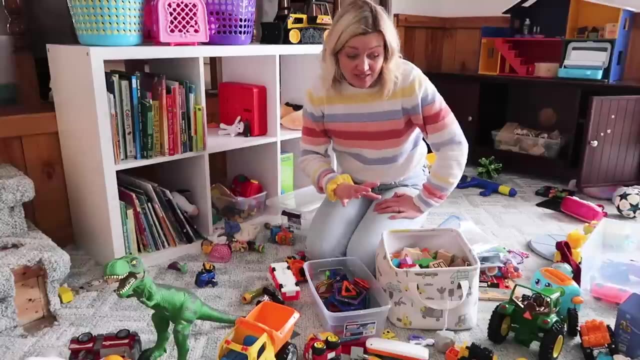 Of like random little cars and random little people, things and balls and all this stuff. And so my kids have all these toys, like they have all these brain toys that are supposed to, like, stimulate their brains. But what I'm finding is, when they have less stuff, their brains are probably 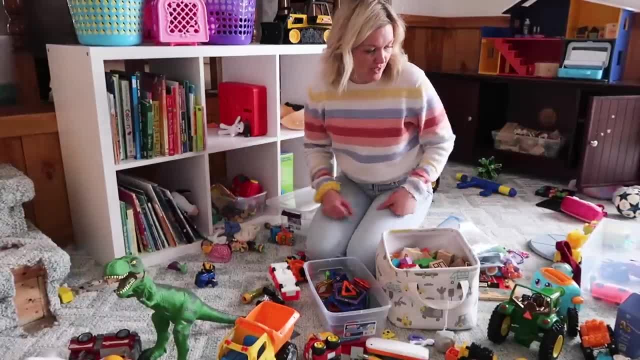 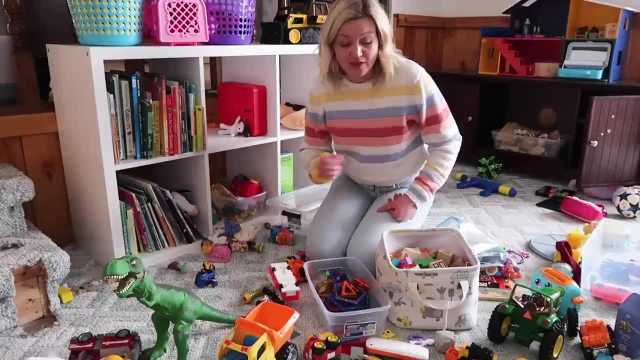 more stimulated because they actually have to be creative and make up their own thing. I don't know anything about childhood development, but I do know that when my kids have just tons of messy toys everywhere, They do not play nearly as creatively or for as long. then if they have just a few things, they can, 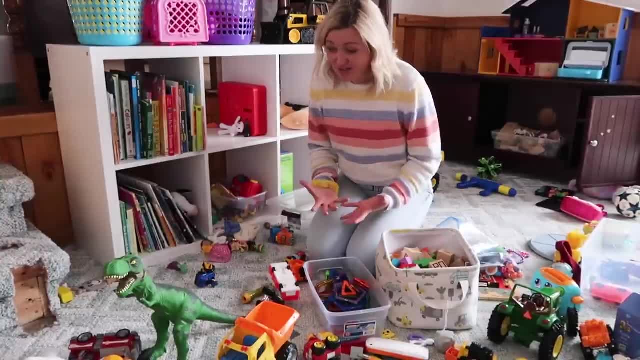 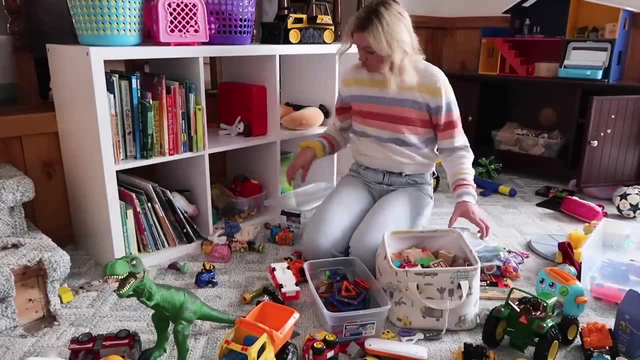 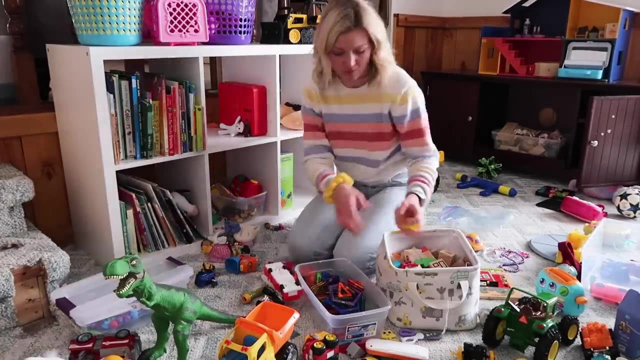 pick from. so it feels bad throwing things away and get rid of toys, but I do know it's better for them, or I'm pretty sure. at least Let me know if you know more about this. Okay, so I'm gonna group the little toys in the little pieces to them. 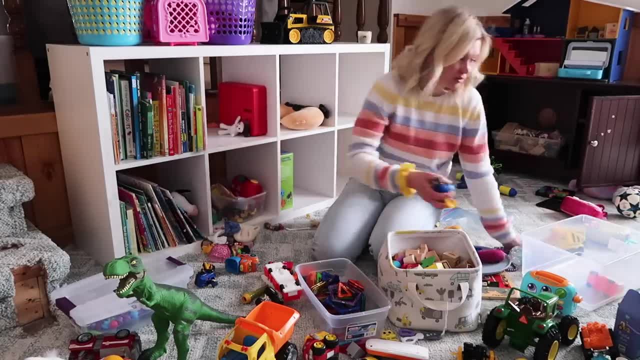 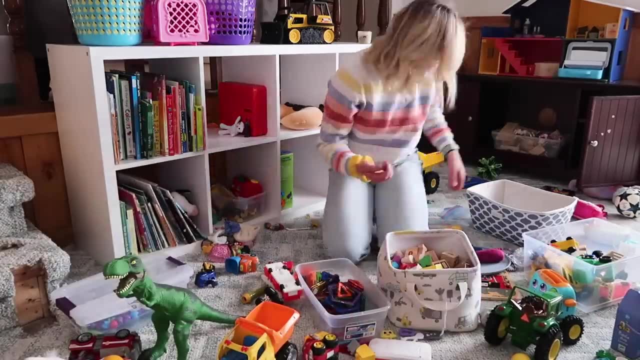 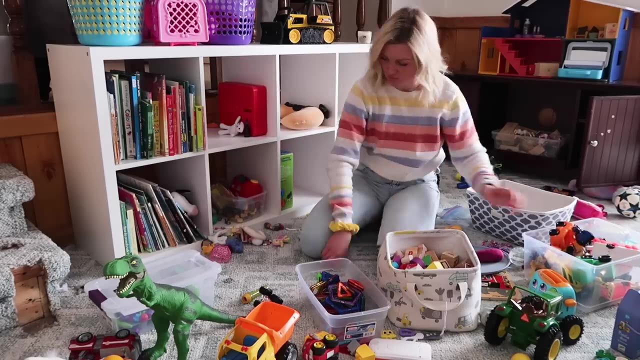 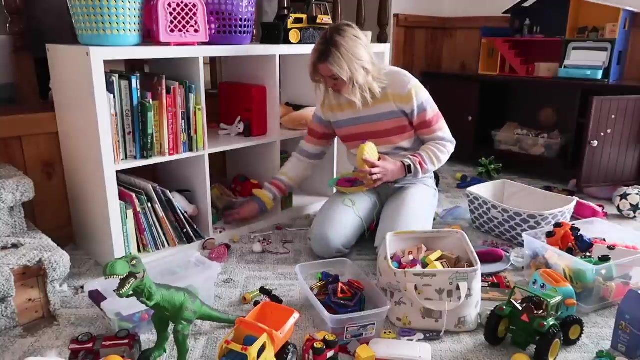 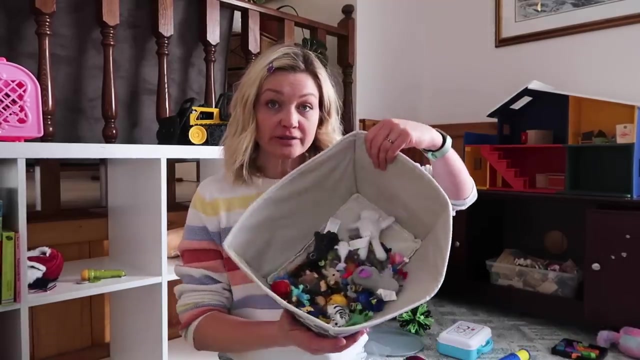 It's time to get ready. Let's go people, and then I'm going to try and cull some of them. All right, so I've got everything basically sorted. We have our little bin of guys. If you've kids, you know what I mean. 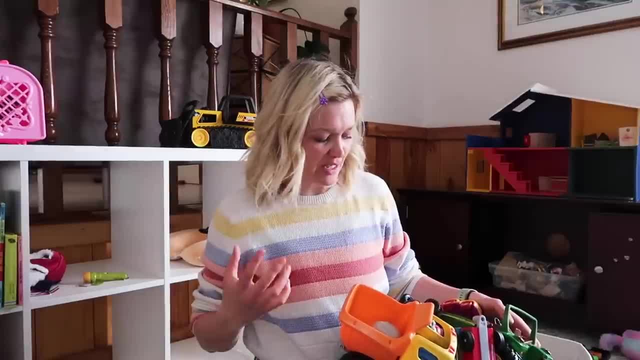 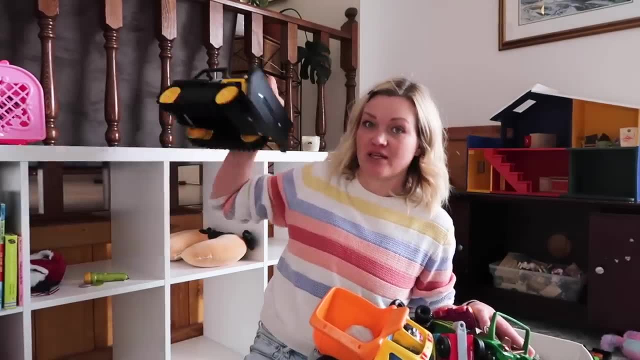 This is our bin of trucks and vehicles. We didn't ever have these, but as soon as we had a boy, people were like: you need trucks. So we've had a lot of trucks come in, in addition to like big things like this. 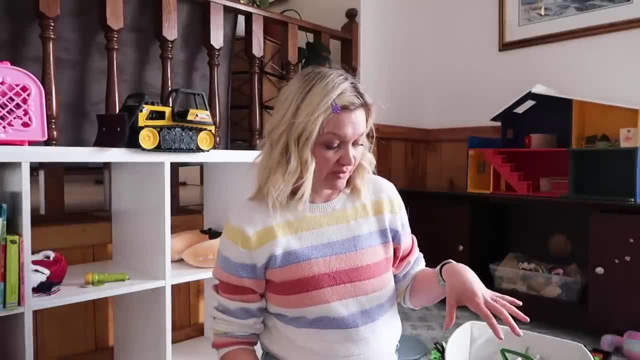 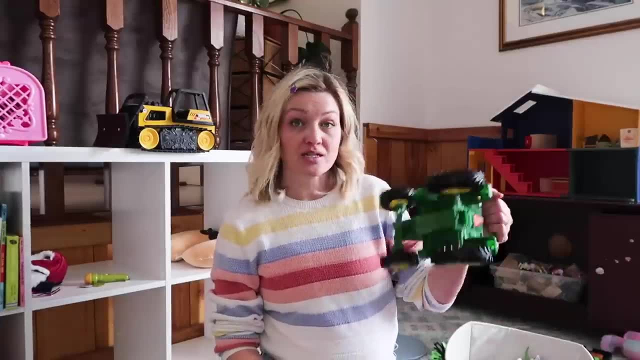 I mean it's like very appreciated, but there's no way one child can play with all of these. So definitely some of these can go to the thrift store or at least away. Some of them can probably go outside, and then we'll just keep the really good ones that. 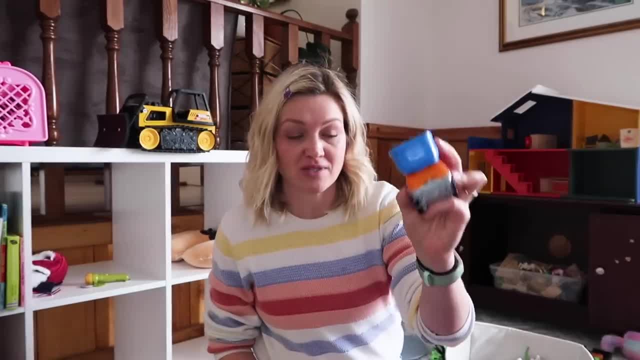 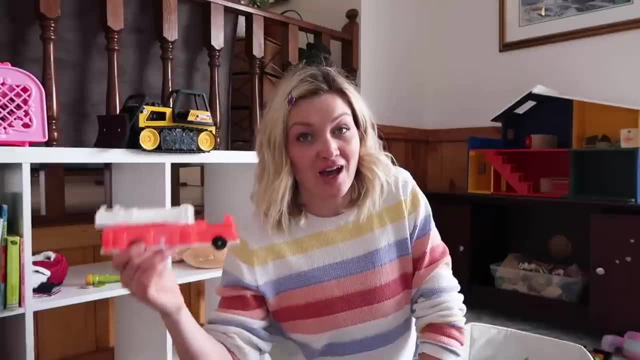 I know he's using a lot. This one never stops singing, So itch We can go. We just have two of these. It's the exact same thing. I confess I'm kind of part of the problem because I'm obsessed with vintage toys like. 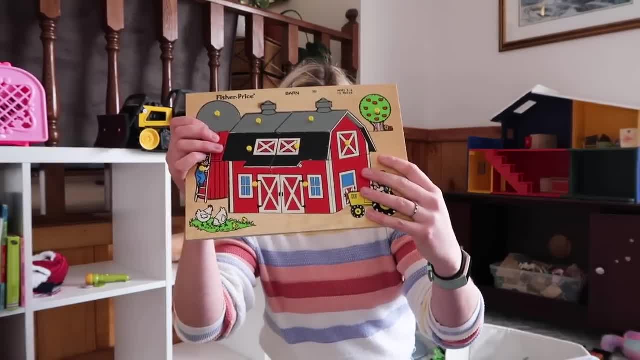 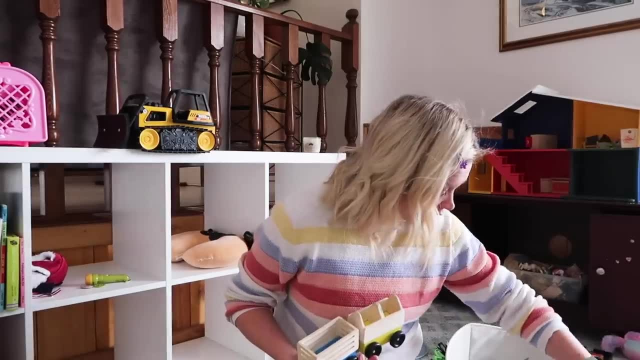 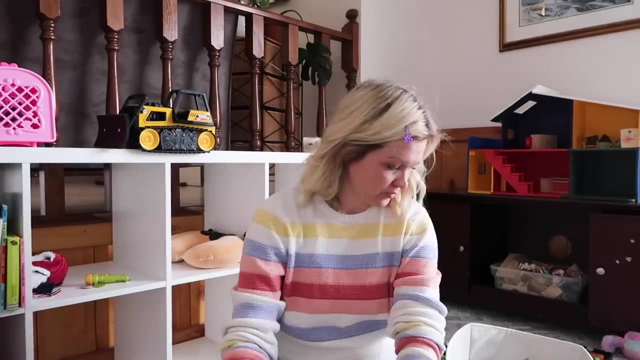 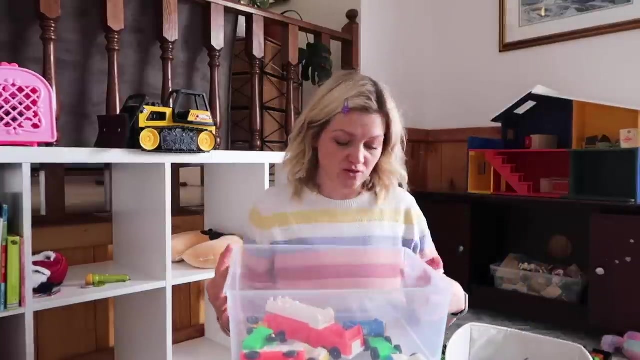 this which is so old: It's from 1971. So it's like 50 years old. This is from 1972,, I think, Be part of the solution, Stephanie. Okay, these are all like our vintage Fisher-Price toys which, at the very least, I want to keep. 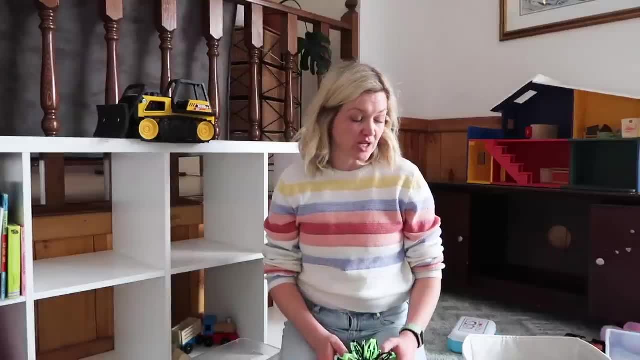 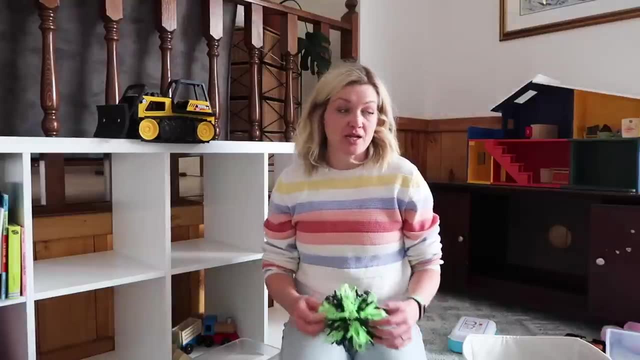 them together, but they do get played with a lot. I reached a bit of a standstill. I'm having feelings of guilt crash over me about getting rid of things and I'm really stuck between- yeah, having my kids have a more fulfilling childhood through creative. 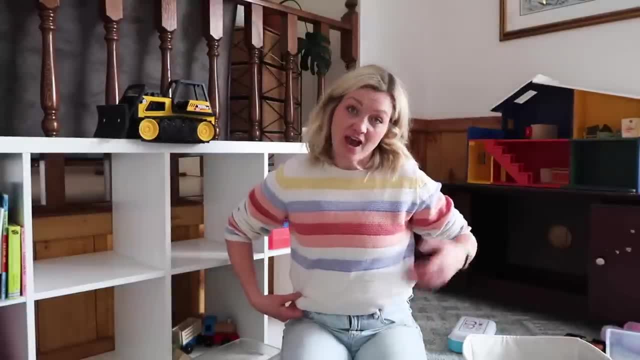 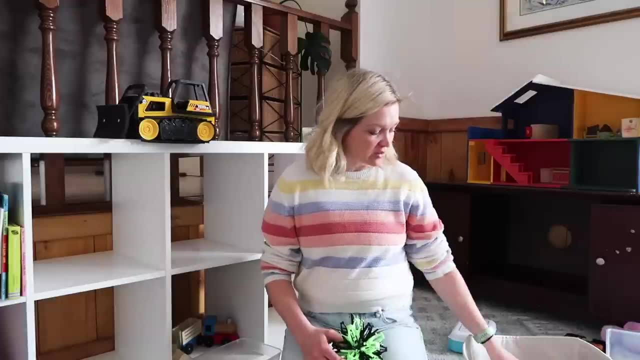 play and not having as much stuff and then having everything they want And me, you know, fulfilling every whim and desire. Oh, this is so hard, Like every little thing I'm like. oh, this McDonald's toy, but they play with it. 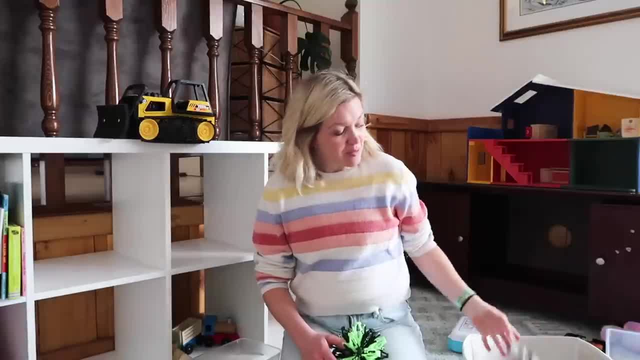 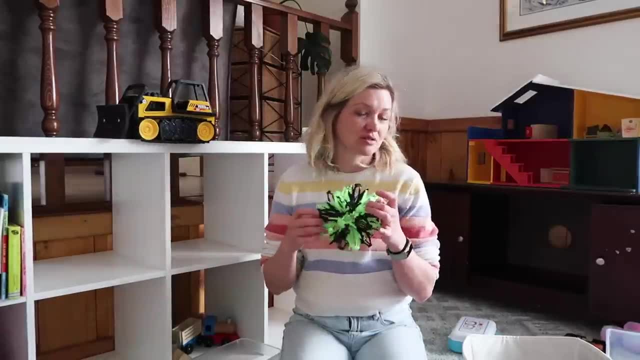 So it's junk, but they love it, So we keep it. but then we can't keep everything. I actually kind of really like this. Maybe I should just keep this one. Well, I'm going to keep this dollhouse. My dad made it for them. 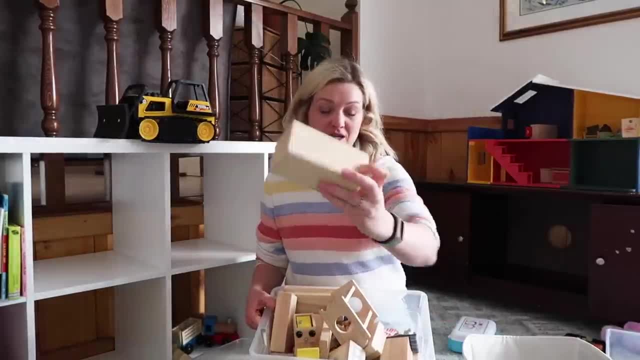 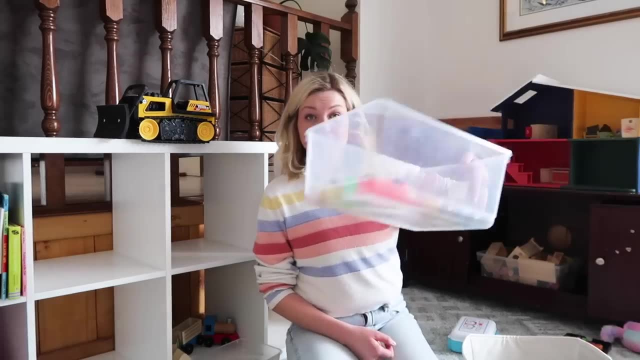 And then we got these really awesome little wooden furniture that he made, and they actually play with this all the time. So I'm going to keep this And just kind of keep it out. My bin of trucks has drastically decreased. I've got a couple more in there like this one and this one, which I know are big hits. 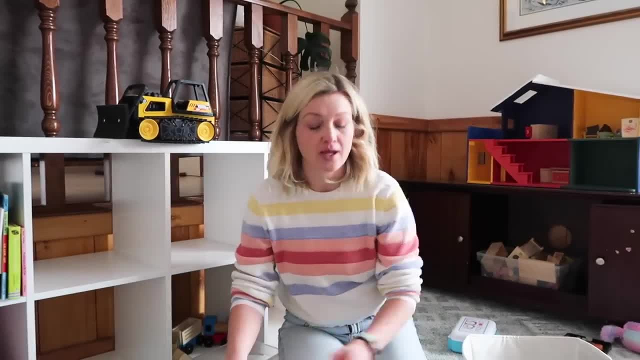 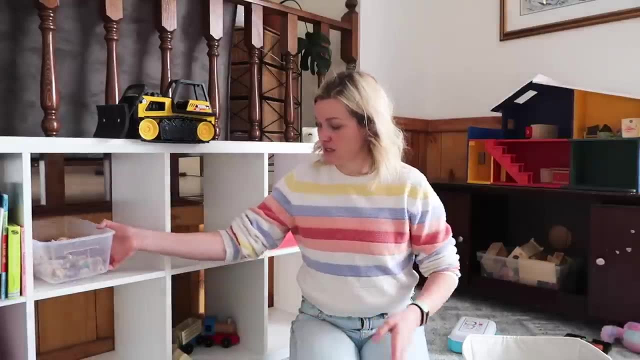 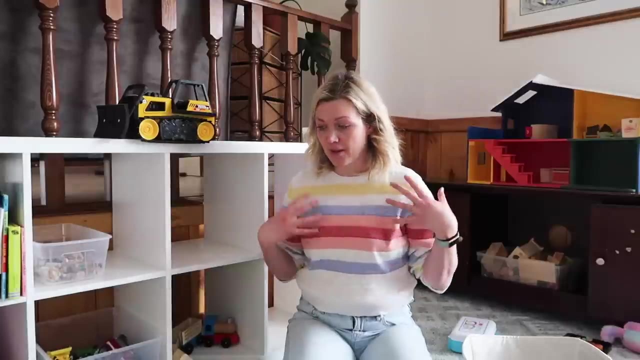 And then I have these little guys, little trucks. So these are like medium sized trucks, giant trucks and then little trucks. Less is more, Less is more. Okay, These little guys can stay out, These can stay here. Not perfect, but I'm making progress and I'm feeling better about it. 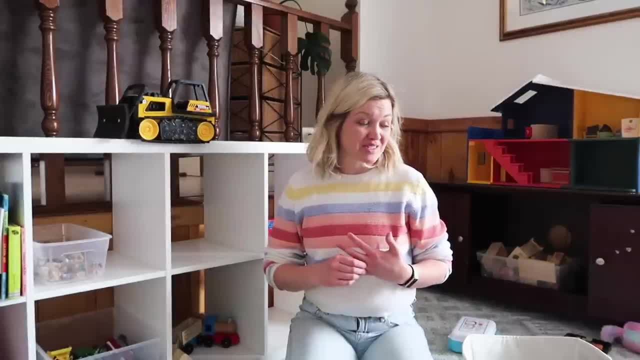 But I I'm going to have to come through this stuff one more time. I think it makes them seriously hard choices. Okay, And then our bin of little guys. I mean, it's not that much stuff, so I'm going to put it in this basket. 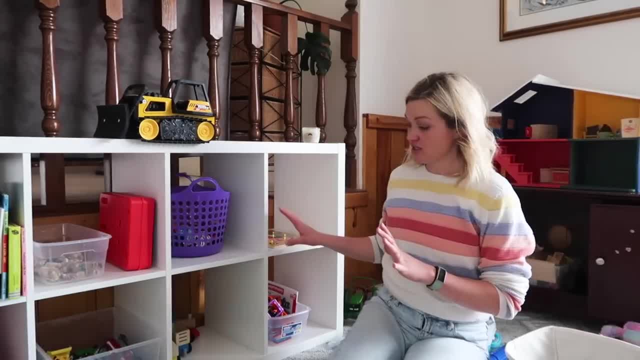 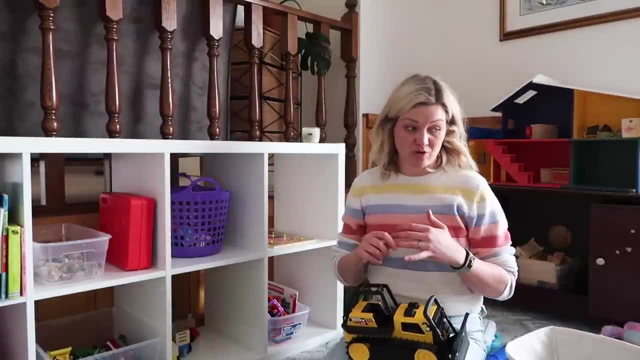 Little bin of things, everything that's not in these shelves. I'm going to pack up the big trucks. I'll keep those out, but everything else I'm going to pack up and either donate or put away. I can't believe. this is where I'm getting stuck. 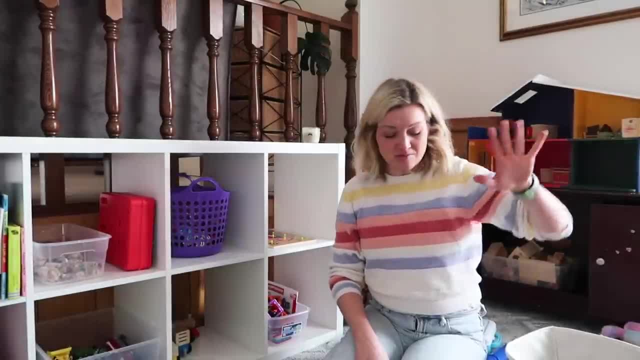 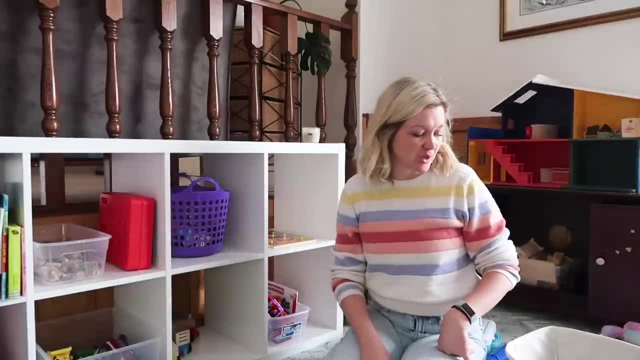 I can't believe this is where I'm getting stuck. but I can't believe this is where I'm getting stuck because I have so many toys. of all things like this is. this has been this is the hardest for me to declutter, because maybe it is because it's their stuff or because I just have so many good memories of them playing with things. but this is not easy, so this is what I'm left with. 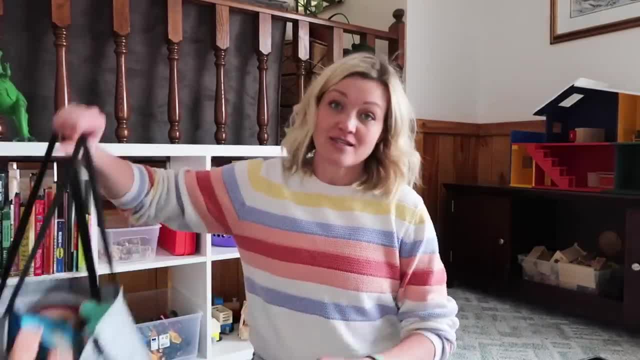 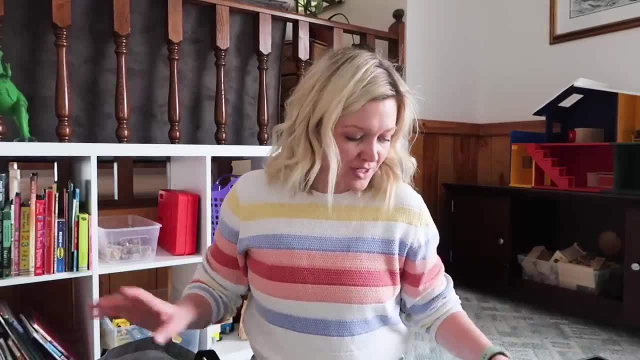 And then I did put some stuff downstairs for toy rotation. This is a bag of stuff to go to the thrift store for someone else to enjoy- all really good, in good shape toys. Just we have too much stuff. a very small bag of garbage. 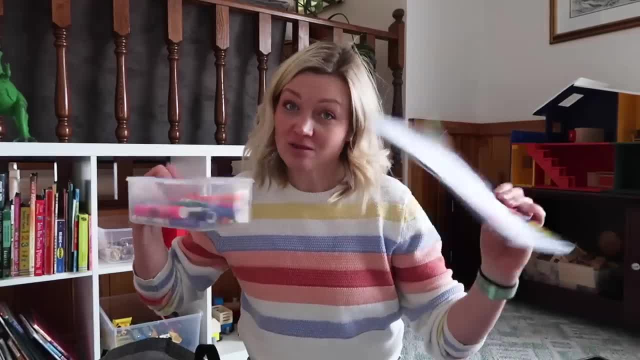 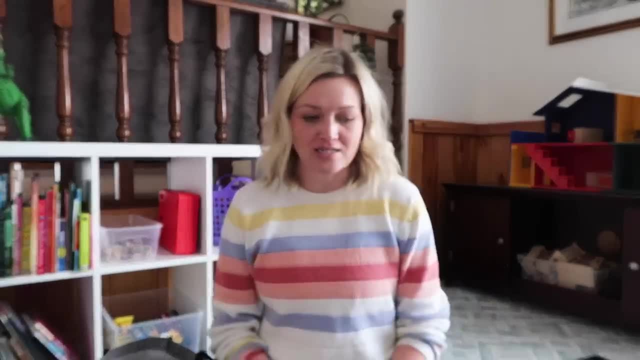 So just broken things and actual garbage. And then I did find a little bit of art supplies kind of mixed in. So I'm going to head over there and clean out some of their art stuff and, yeah, just tidy it up. So it's nice and easy to use. 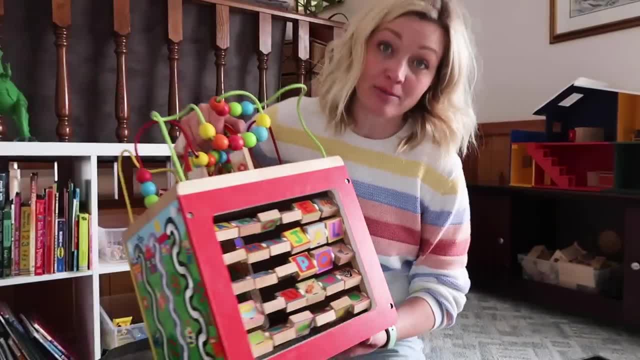 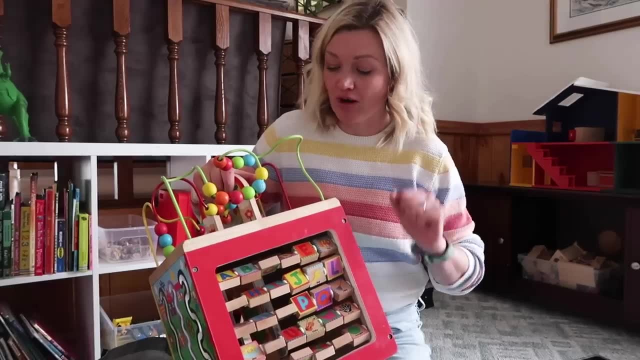 Oh, one more thing. I'm going to get rid of this guy. This guy has not been touched in so long. I already declared it once and then my children drug it out of the garage, brought it back in here, and they still don't play with it. 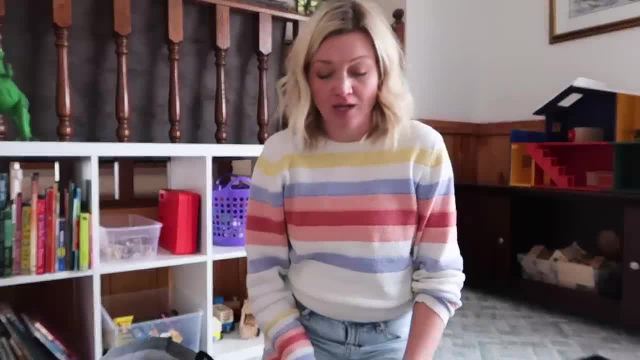 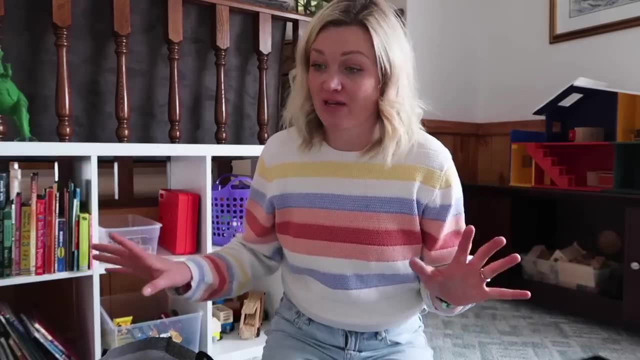 So last chance it's gone. Oh, I swear, Nothing makes a toy more interesting to play with. Then Throwing it away suddenly It's the most fabulous toy we can't imagine living without. Anyways, let's move on. art stuff. 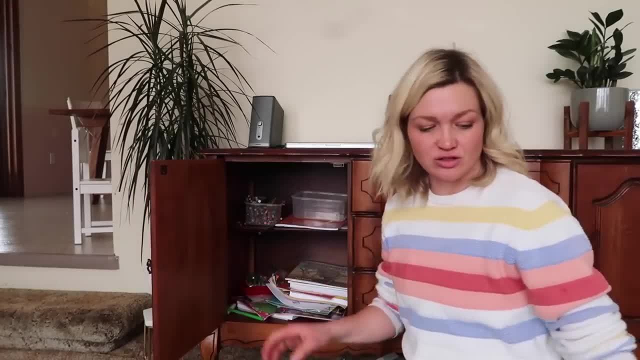 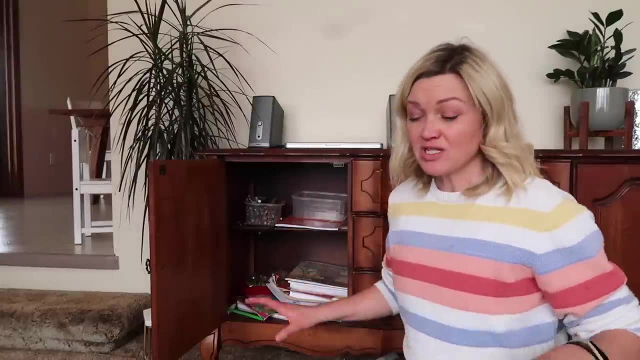 So this is where we keep their art stuff, and it generally stays under control. I also have this random bin of stuff that I've collected all over the house, So I'm just going to quickly go through things. We're mostly at the place where we're just drawing on paper. 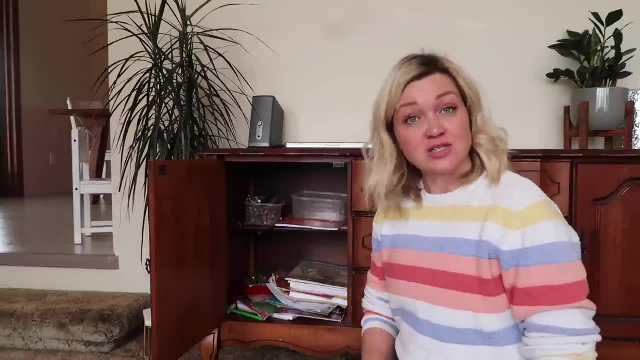 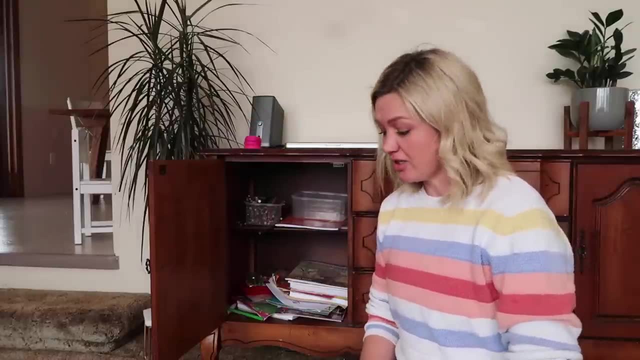 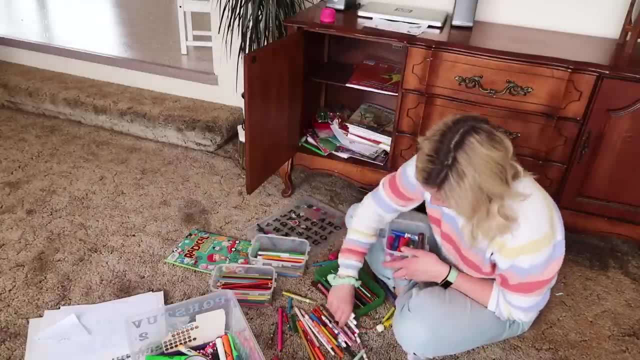 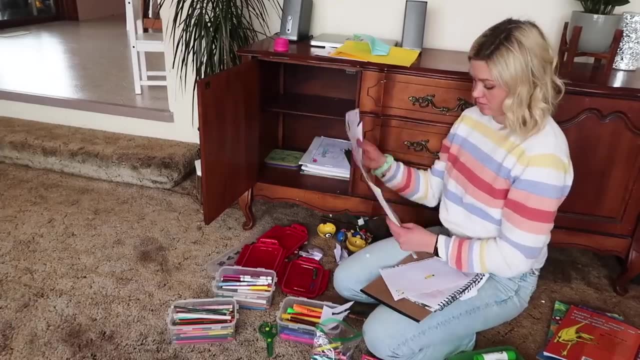 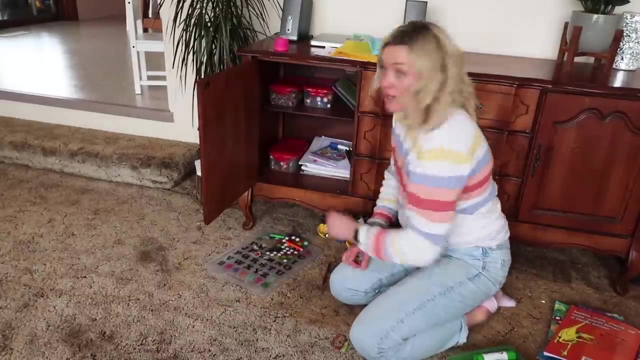 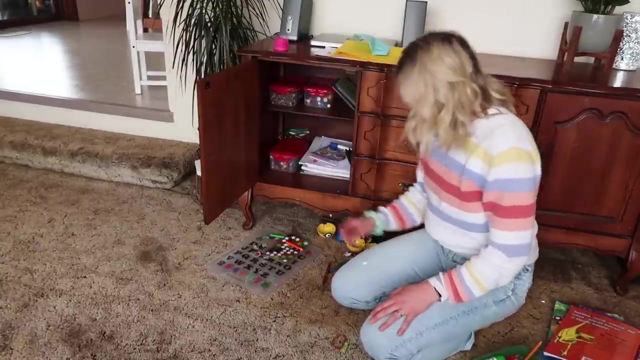